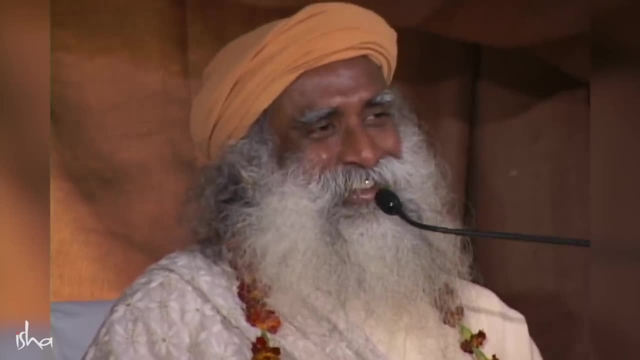 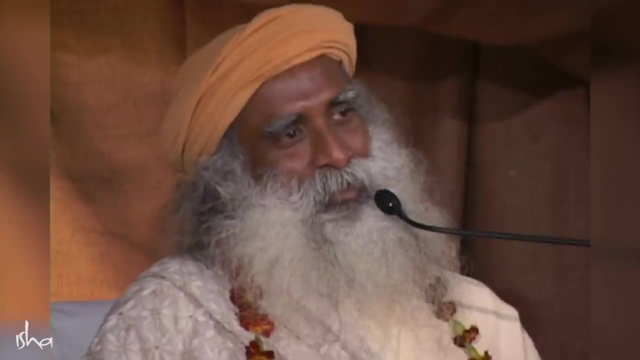 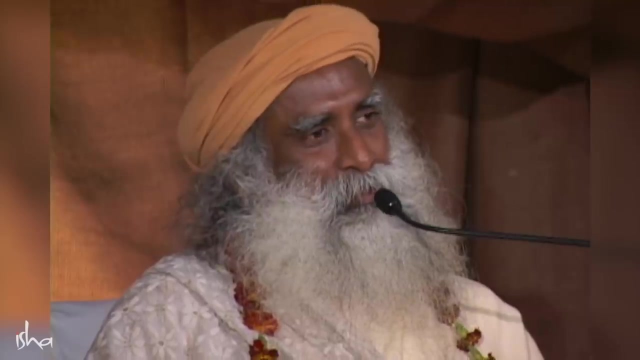 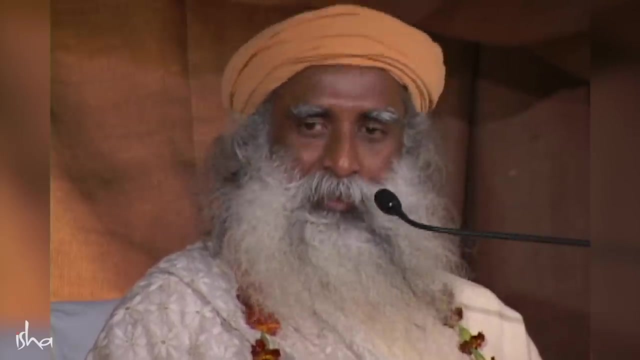 I don't think I am. You can't make a fool of yourself, nor can you make an intelligent one out of yourself, isn't it The way you are? it's the way you are Now in trying to be smarter than what you are. 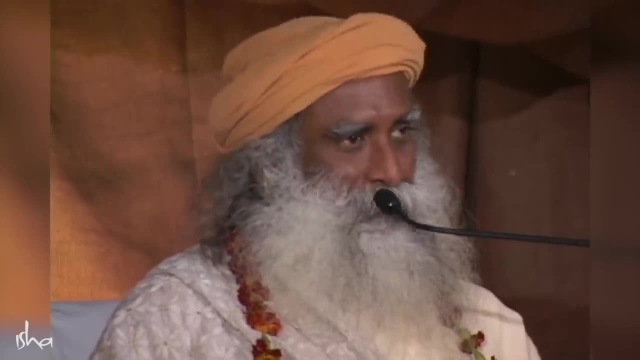 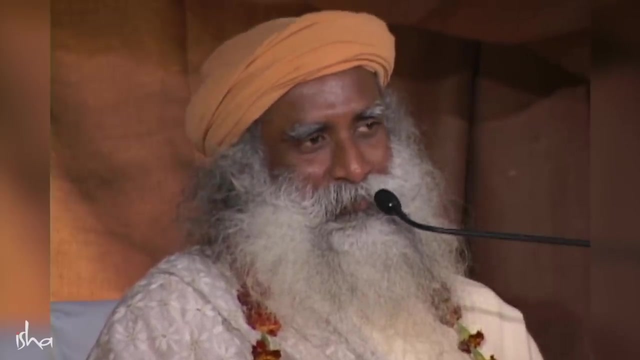 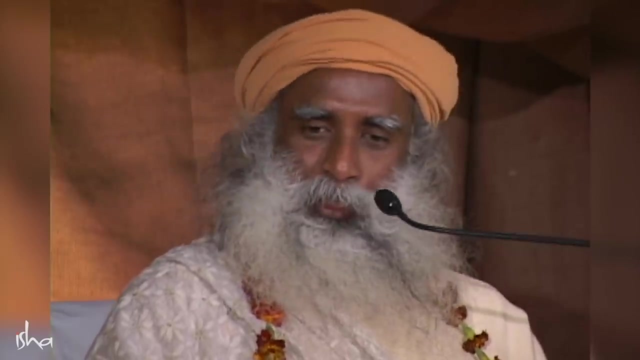 that's when you make a fool of yourself. You are generally not so hard upon yourself if there was no public watching you, Isn't it? That's the whole thing. If there is nobody watching you and you make a fool of yourself. 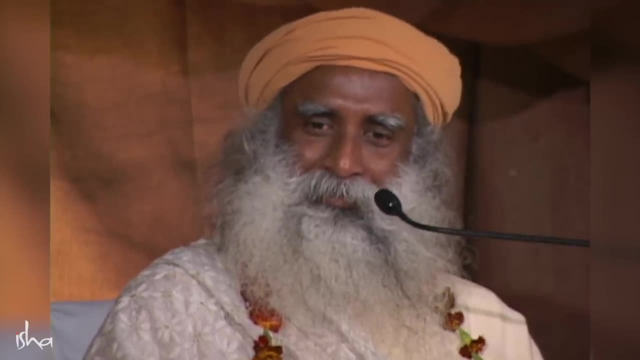 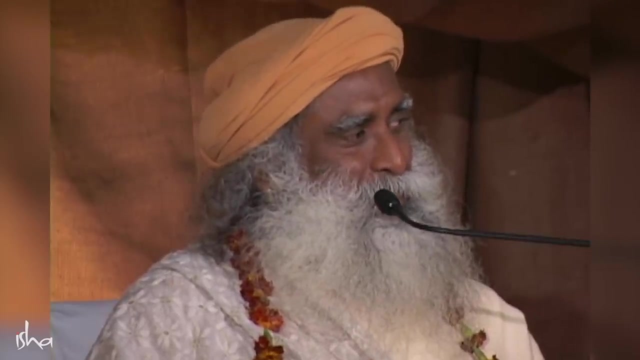 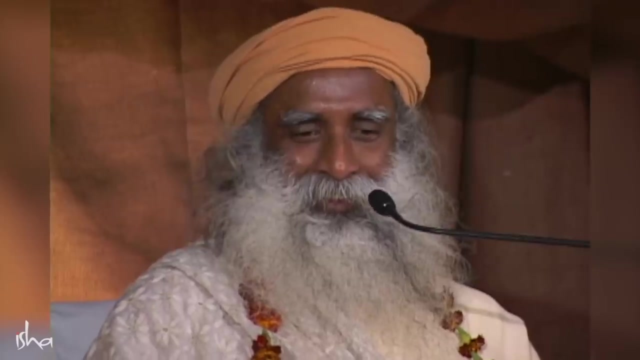 you are not hard on yourself. You are very pardoning, isn't it? Yes, Ten people were watching you, and now the message of your stupidity is going to spread around the world. That's what is bothering you. No, your very stupidity should bother you. 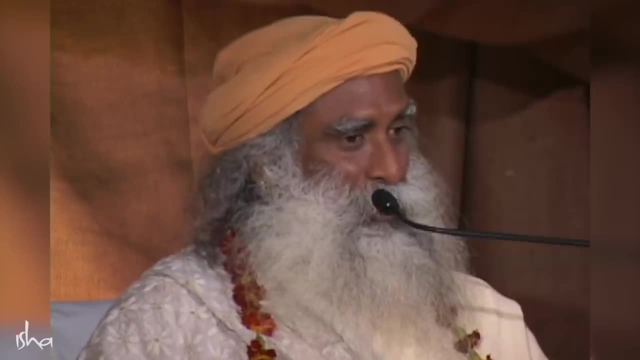 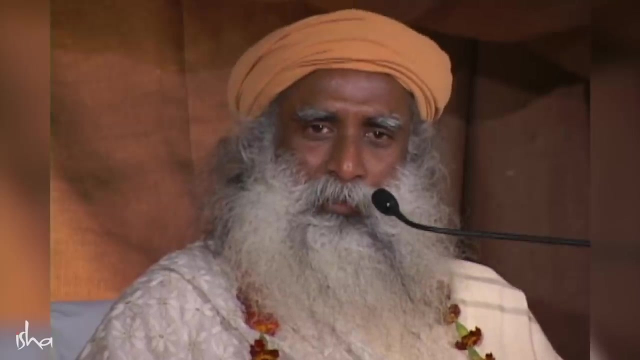 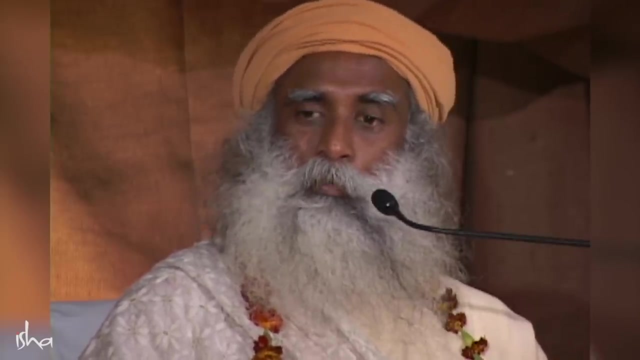 Not the publication of your stupidity. Your very stupidity should bother you. That's when you will turn spiritual. It's not about what people think about you. You are foolish with so many aspects of life That itself bothers you, Not because ten people are watching you. 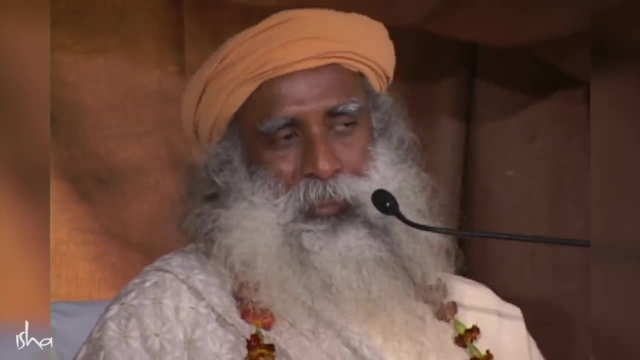 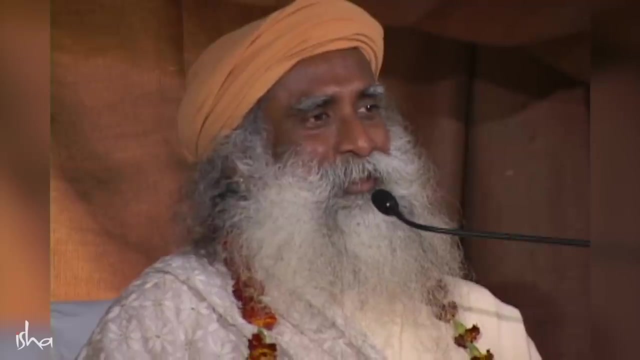 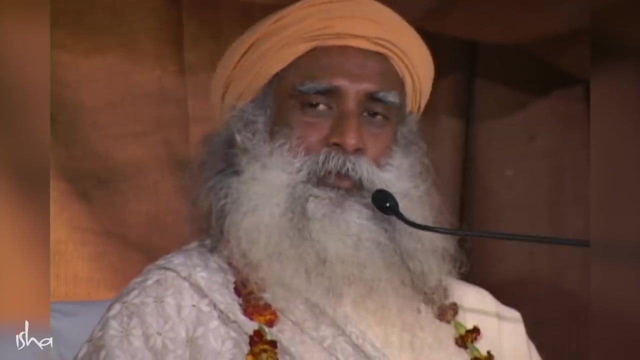 When that happens, you will naturally turn spiritual. Now you are only concerned about in front of ten people. it happened. I think it's good. A revelation is happening. Now why are you doing public speaking? I think it's good. 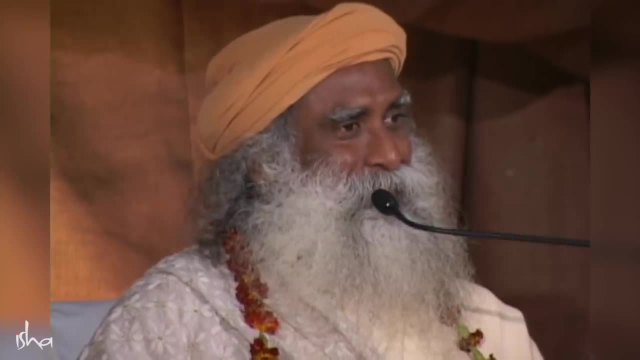 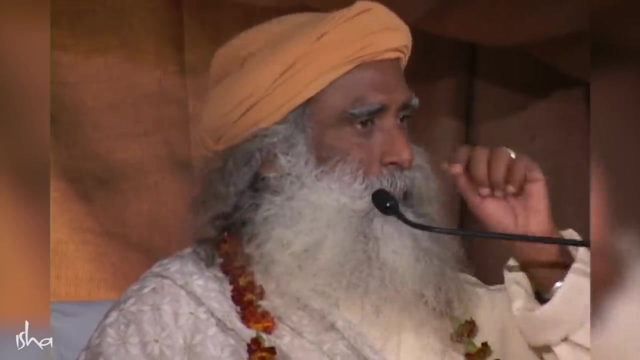 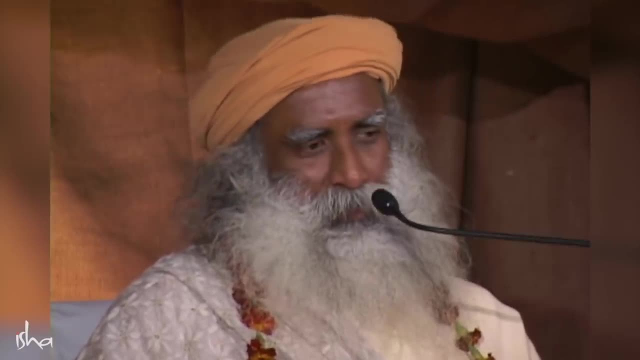 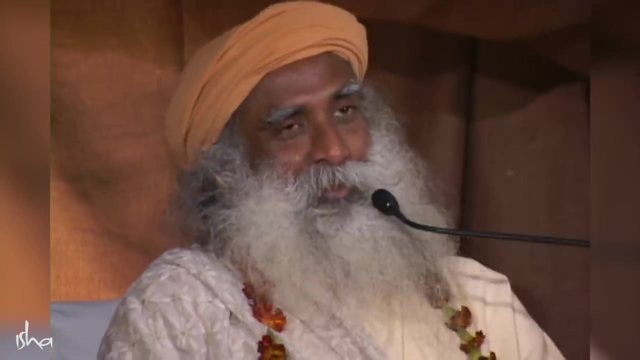 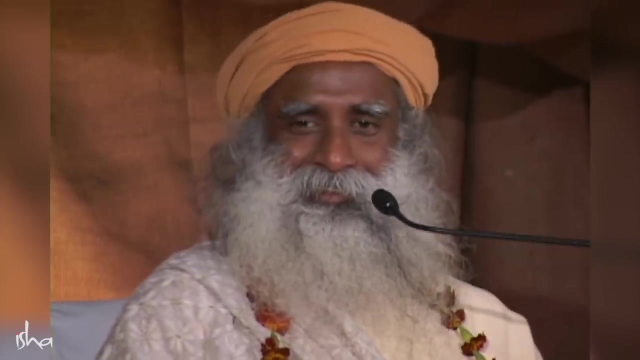 You don't do any public speaking, You just speak. People always say, No, I am not used to speaking into the microphone. Tell them: don't speak into the microphone, You just speak. Microphone knows what to do. Why should you speak into the microphone? 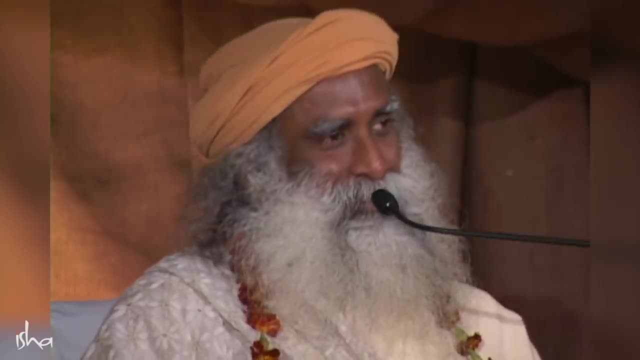 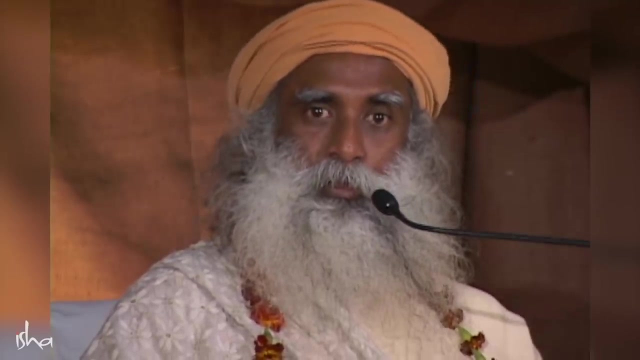 You simply speak. Microphone will do what it has to do. You simply speak. Microphone will do what it has to do, Isn't it? And why are you doing public speaking If there is public sitting here? If there is public sitting here, 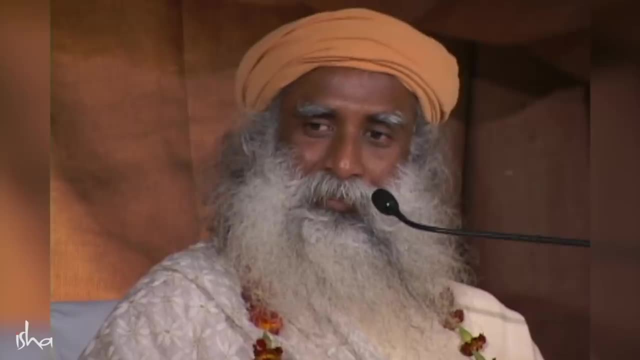 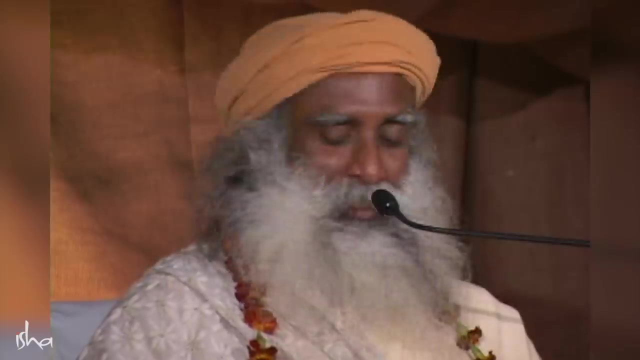 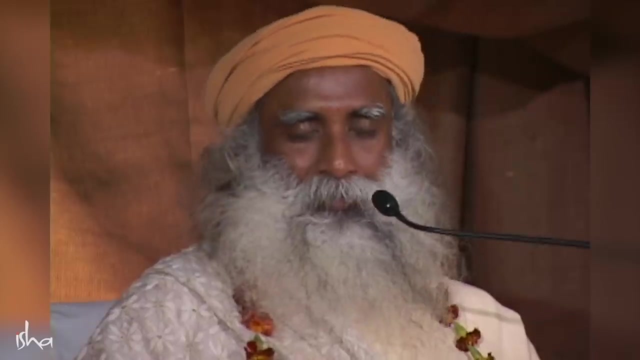 naturally you will be. naturally you will be. You know, there may be somebody who is going to pull you down out there. I was recently, or eight, ten days ago, I was with a group of people in New Delhi. I was with a group of people in New Delhi. 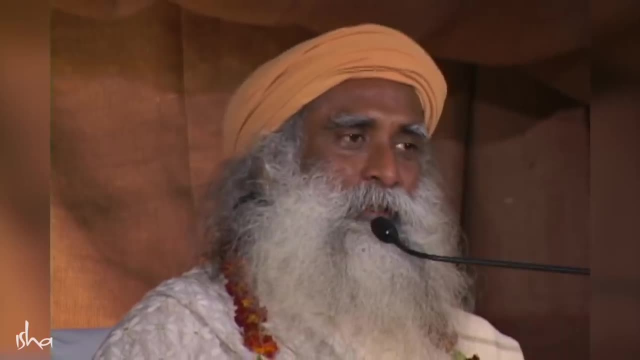 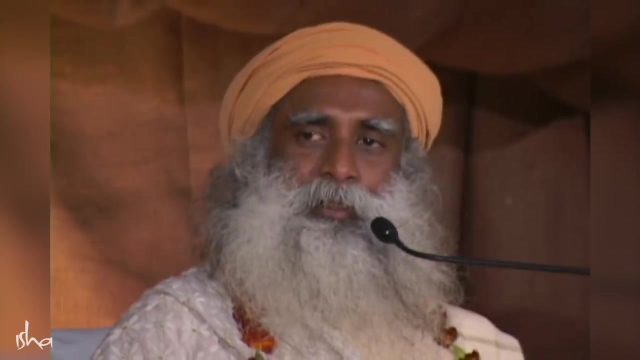 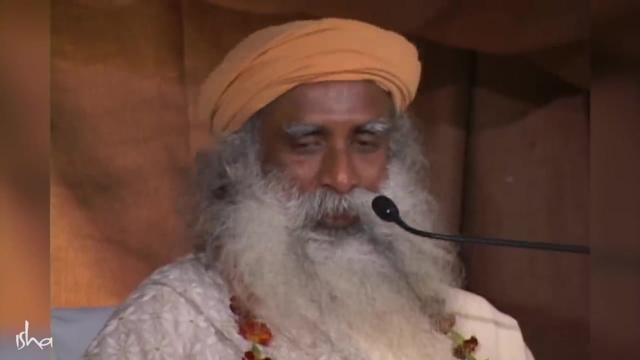 I was with a group of people in New Delhi. This person- now he is a little out of action, but he was at one time. he was at one time the Prime Minister's right hand man and he was a minister and he played many roles. 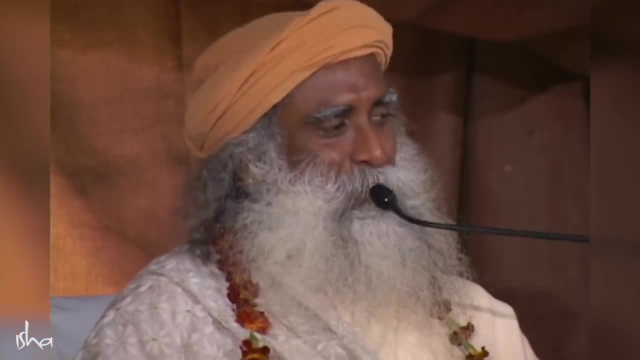 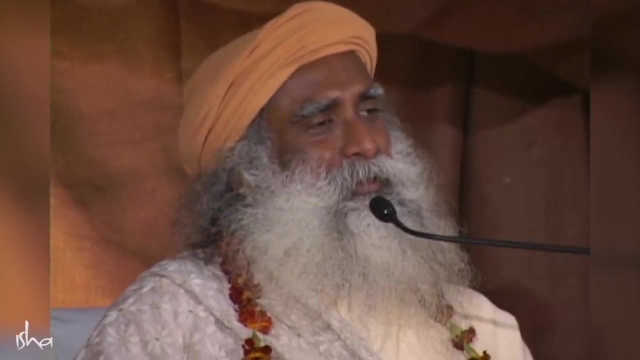 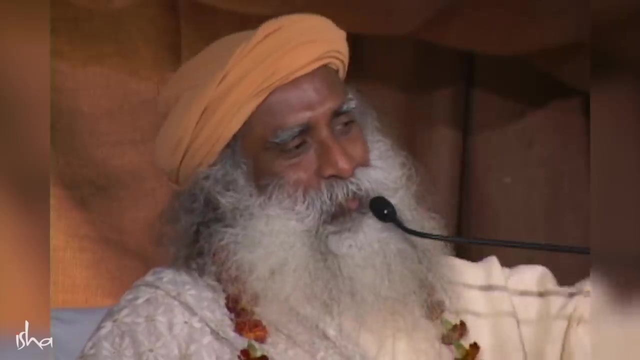 He has gone around the world, spoken to any kind of and every kind of group in the world. We were just talking about something and he said: even I know this much: he has been with some great leaders in the country, like Indira Gandhi. he has been next to her. 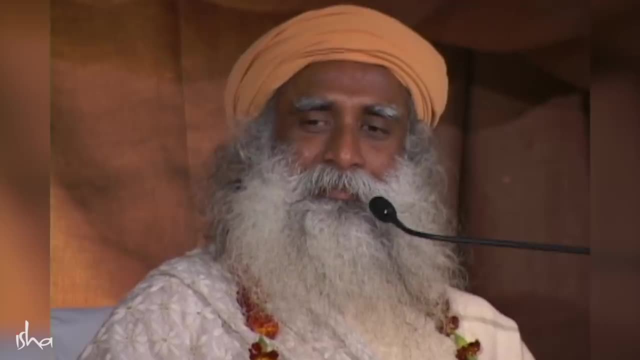 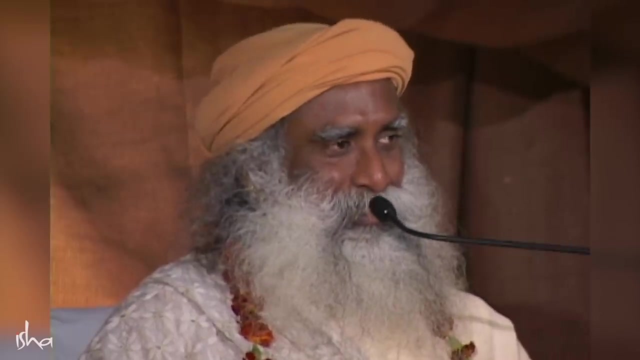 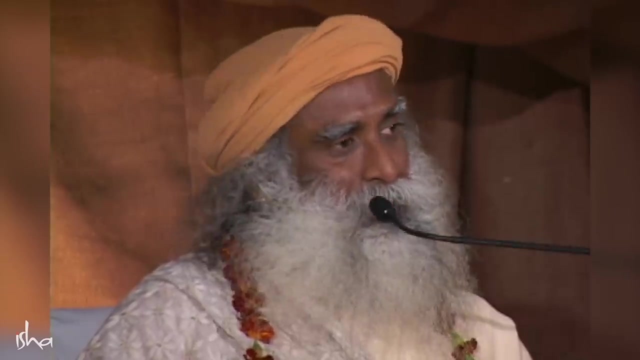 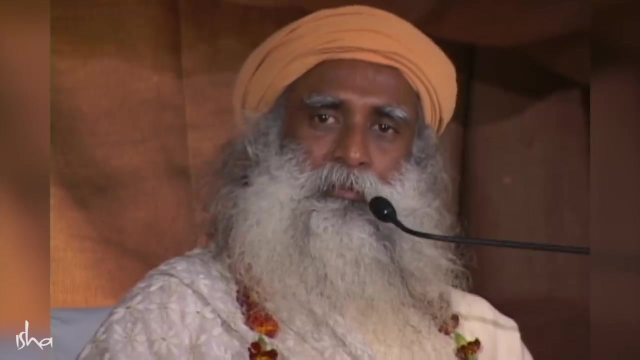 right through her power stage and he said: the greatest leaders: when they first stand in front of a crowd, there is a little bit of nervousness. After that they become okay. I said this nervousness is happening to you because you claim that they are a part of you. 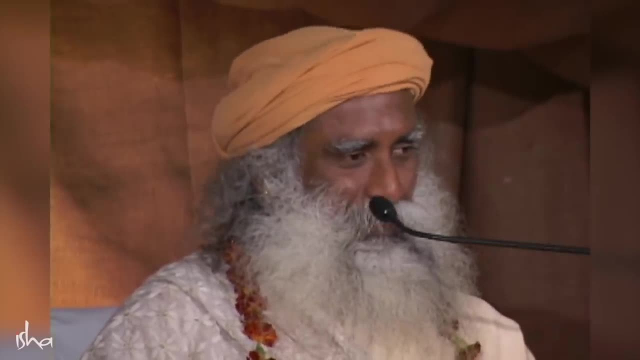 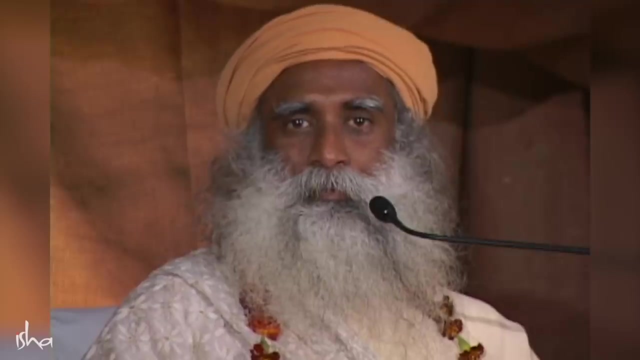 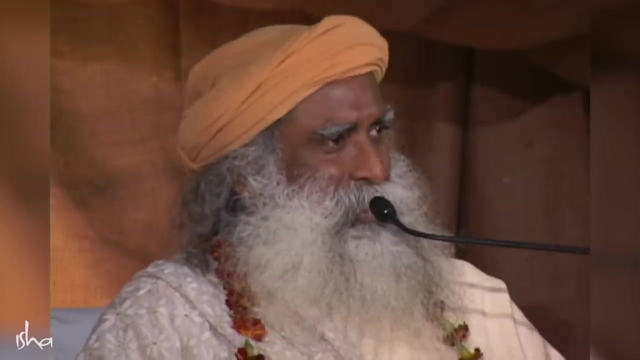 but it is not true. That's why it is happening to you. If you truly saw that this is all a part of you, that this is all a part of you which is talking to yourself, which is talking to yourself, where is nervousness? You can say anything you want. 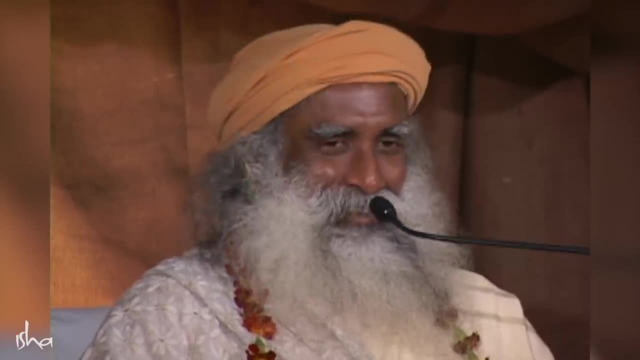 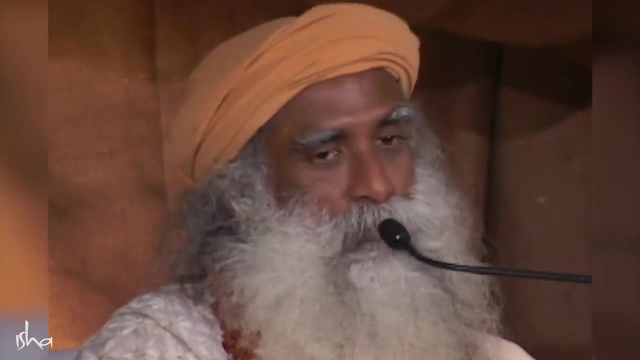 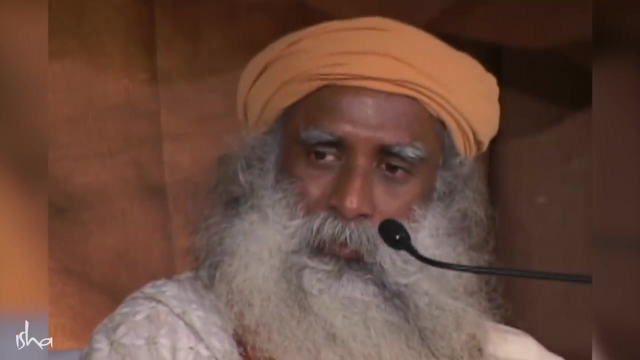 Do you see? I just say whatever I please, So you don't do any public speaking. If you truly hold everything as yourself, you simply express what is true with you, and that's all. Why would you be then? why do you have to beat yourself?